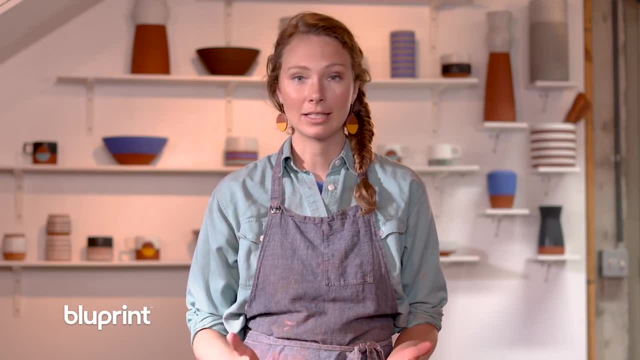 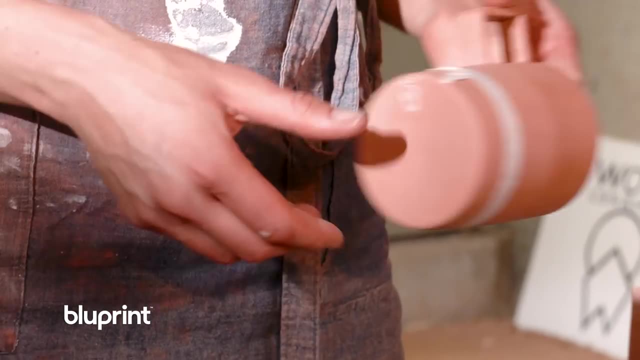 to glaze? Have you waxed the parts where you don't want any glaze to land, or have you put tape around it? Think about how you're going to hold it in your hand while you're glazing, just to make sure that everything adds up. 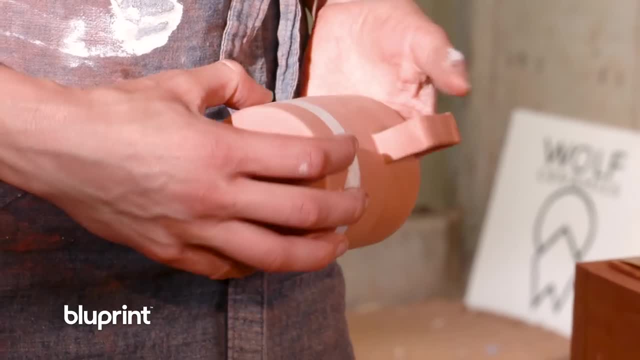 I'm going to start off by glazing a simple white muck To ensure that I have a straight glaze line around it. I'm going to start off by glazing a simple white muck To ensure that I have a straight glaze line. 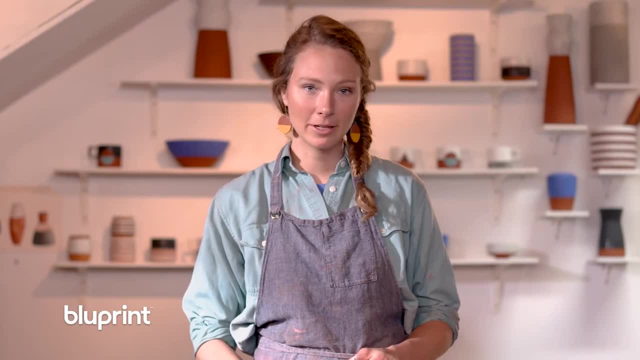 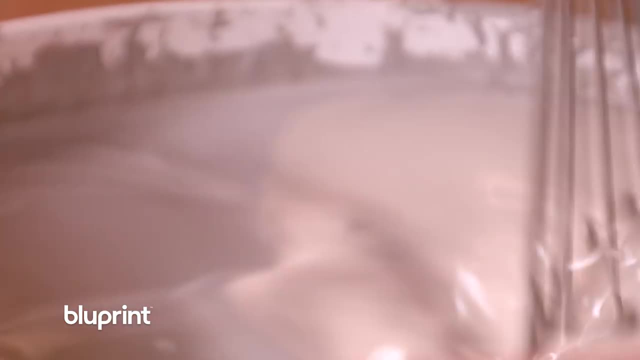 around the bottom. I've just put a piece of masking tape around it Before I dip it in the glaze. I want to make sure that my glaze is really well mixed. I'm going to mix for a while, scraping the whisk on the bottom of the bucket, making sure that there aren't. 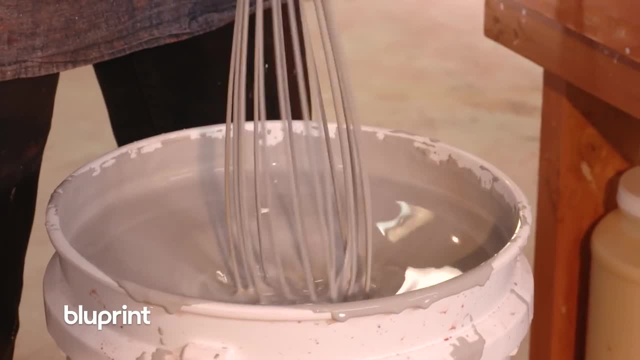 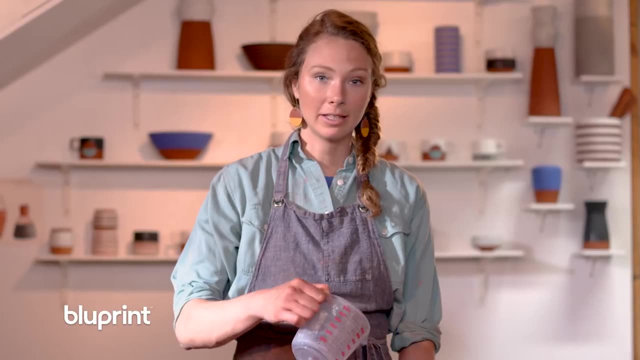 any chunks floating around. I'll be using a pitcher to glaze the interior of the mug, so I'll start by filling the pitcher, filling the mug, and as I pour the glaze out of the mug, I'll swiftly continue on to dip. 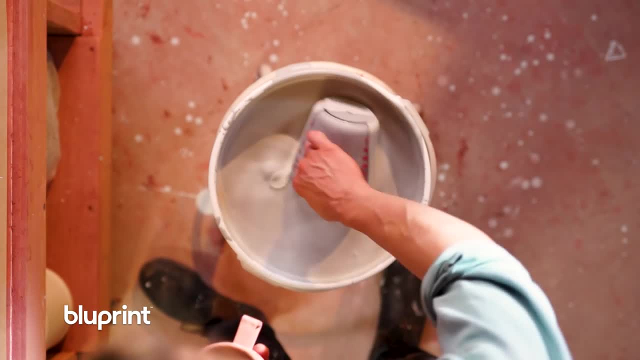 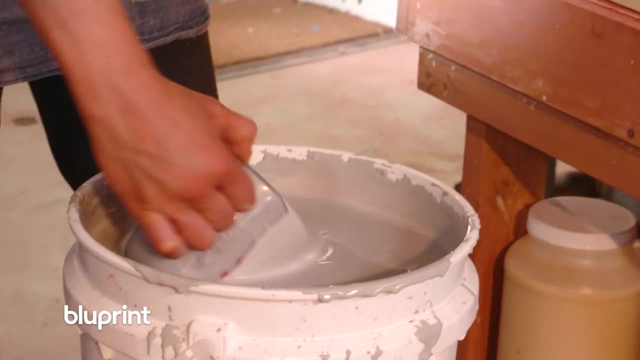 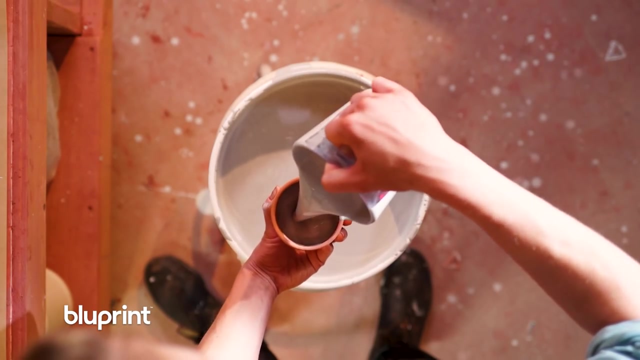 the outside of the mug in the glaze. Here we go. I usually like to just make sure there aren't any big chunks floating around. get a hang of my pour. I'm rotating it, dipping it to the tape and now I'm going to give it. 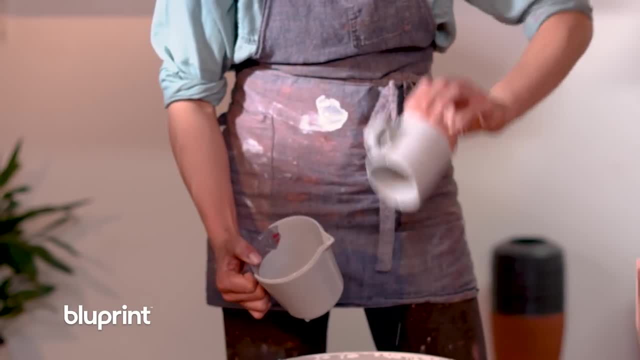 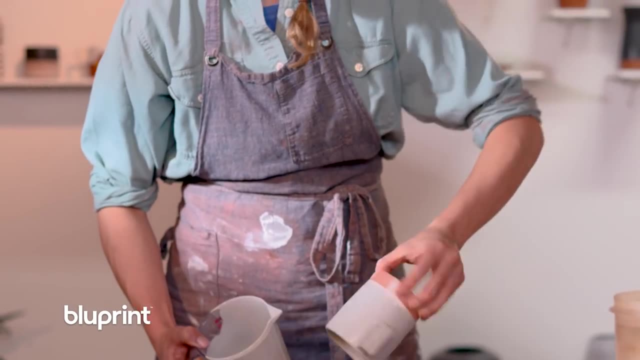 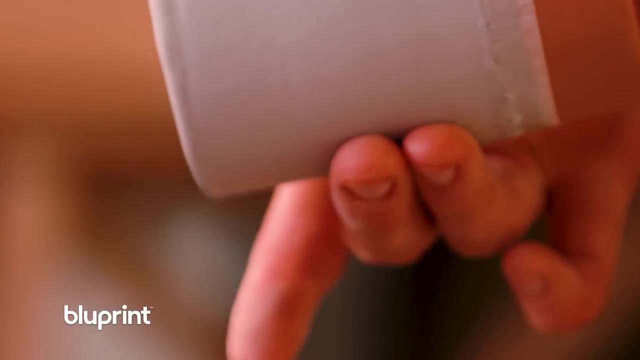 a shake just to make sure there aren't any big drips As I shake it. I'll just make sure that I continue changing orientations of the mug so that there isn't glaze globbing up on one side of it. As you can see, the glaze has dried very quickly. I can already hold my mug So I can clean. 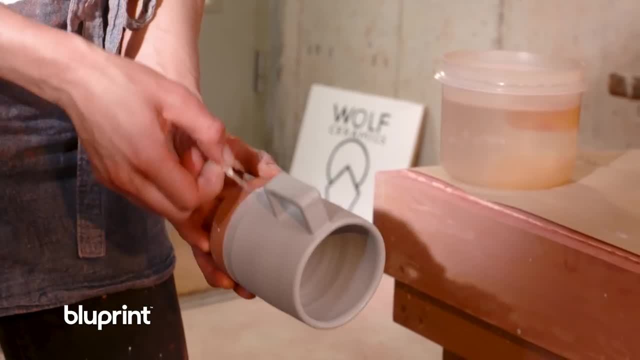 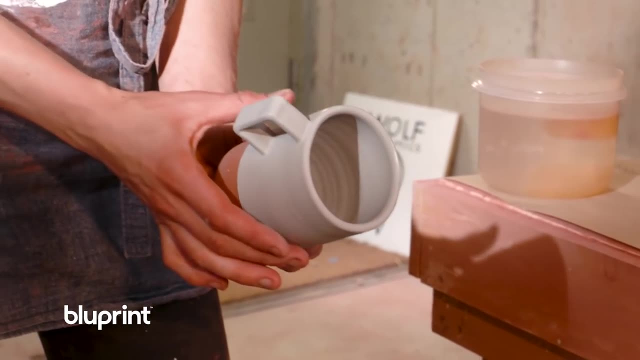 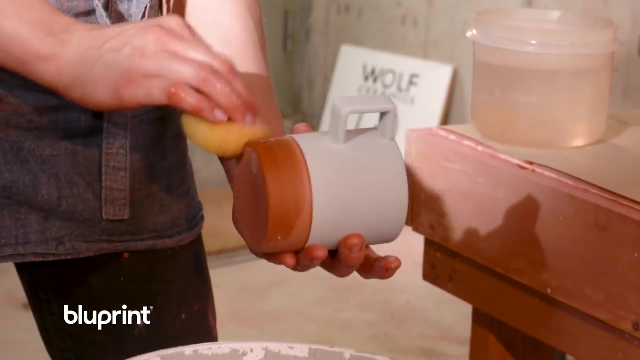 up the glaze at the bottom in just a moment here. but I'm going to go ahead and peel away my tape And now I'll use a sponge, And now I'll use a sponge And I'll just clean up any drips that landed on the bottom. 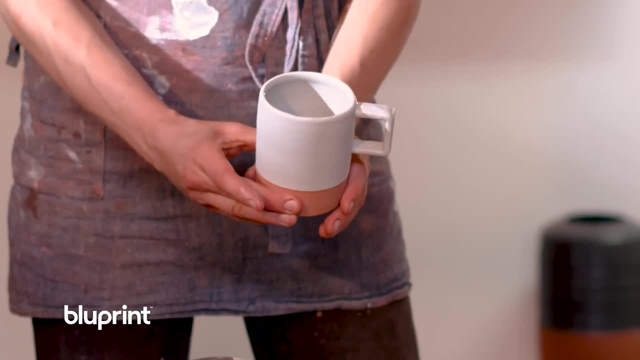 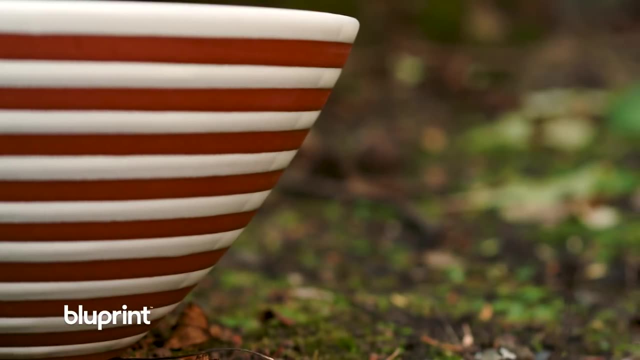 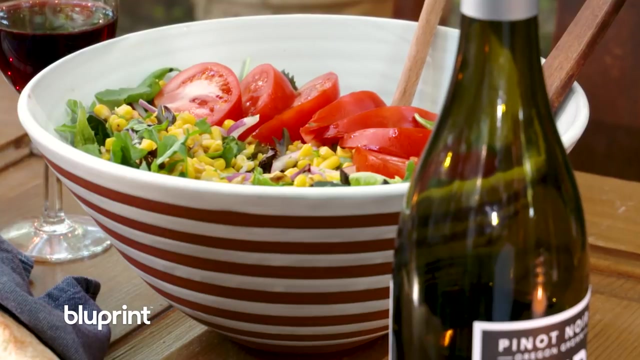 I'm also just kind of smoothing out that glaze edge, since it's a little ragged in places. My mug is ready to go on. the kiln Wax is a great tool to use to add really simple design elements to your piece. I like it because 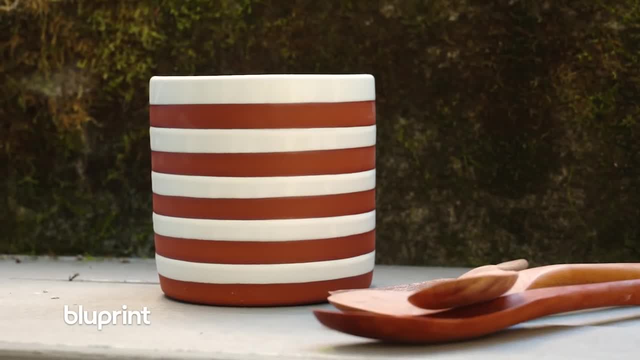 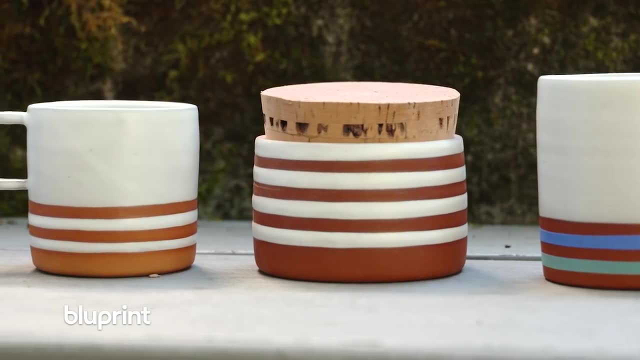 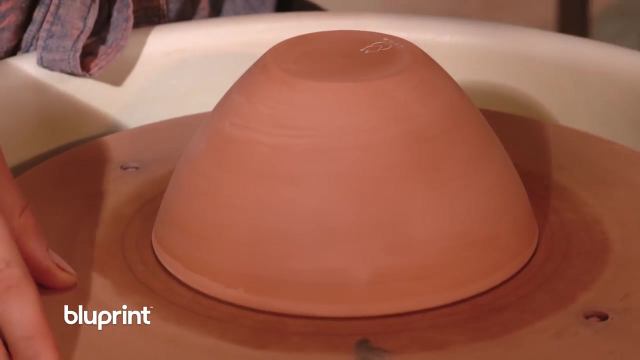 it enables me to play on the contrast between the color and texture of the raw clay and the white glaze that I'm using. It enables me to make contemporary designs that are still simple enough to fit into a classic and timeless aesthetic. So I'm going to start by making stripes on this bowl, And again, there are tons of options. 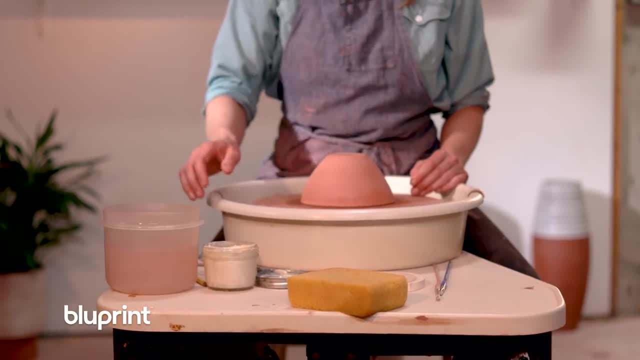 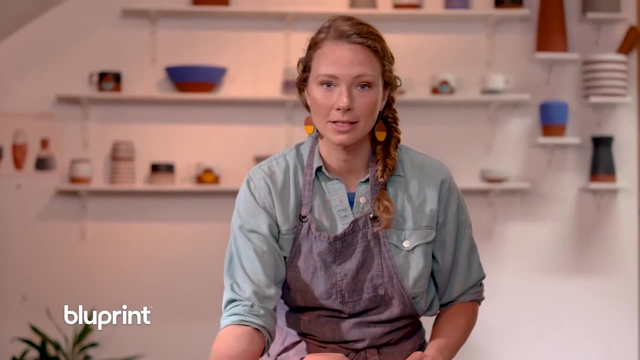 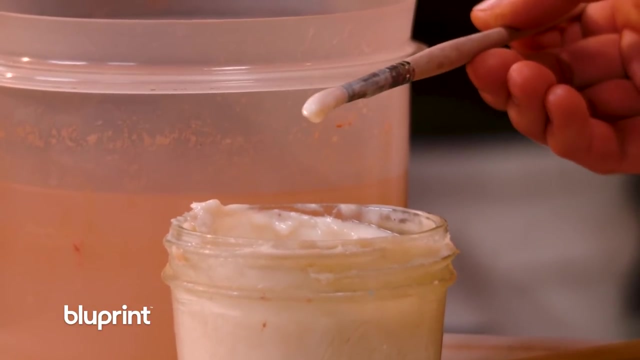 and tons of different ways that you can use this material. I like to use reed wax. Reed wax is this water-soluble liquid wax that actually dries into a water-resistant substance after drying, So it's really, really useful. It's also a little tricky to work with at times because 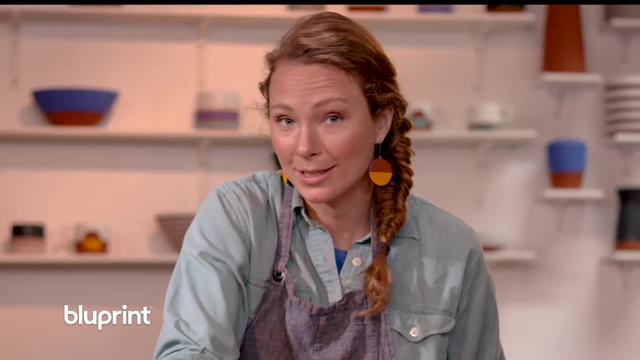 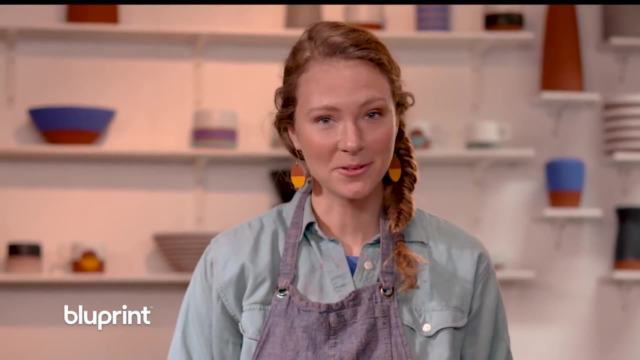 if you get it on your clay in any spots where you don't want wax to be or any areas where you'd like to have glaze later, it's really hard to get off. So it's very useful. but you just want to be sort of slow and gentle and careful when. 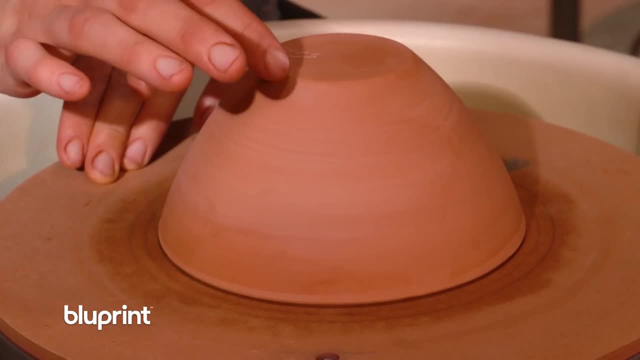 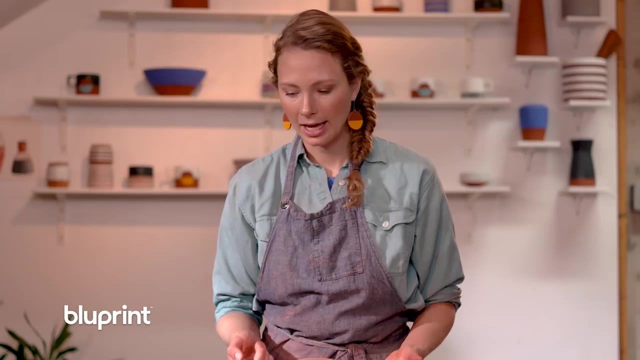 you're putting it on. If you drip it down the side of your bowl, then you will have a line where glaze won't stick later. So on this bowl I'm going to paint stripes with reed wax And I like to just map them. 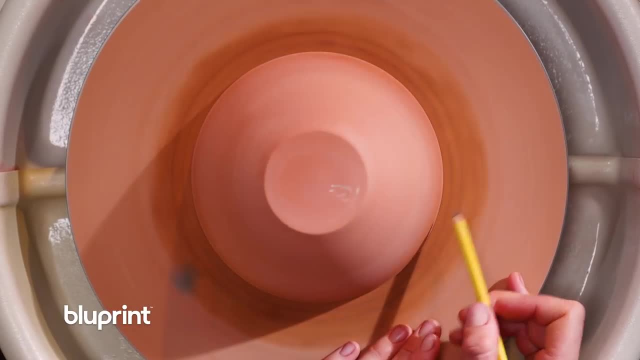 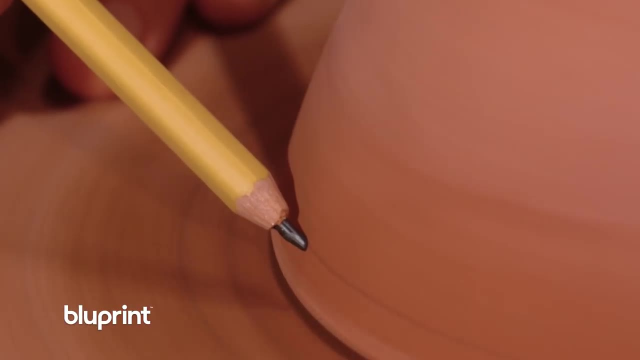 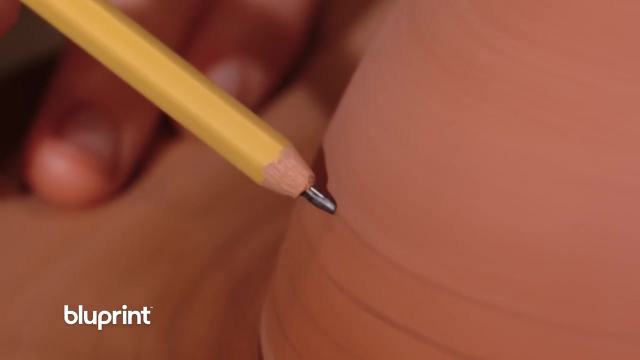 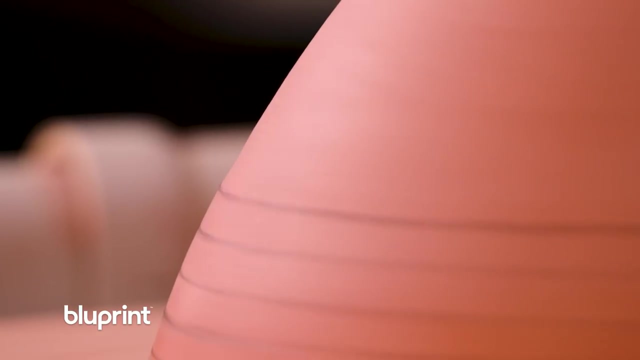 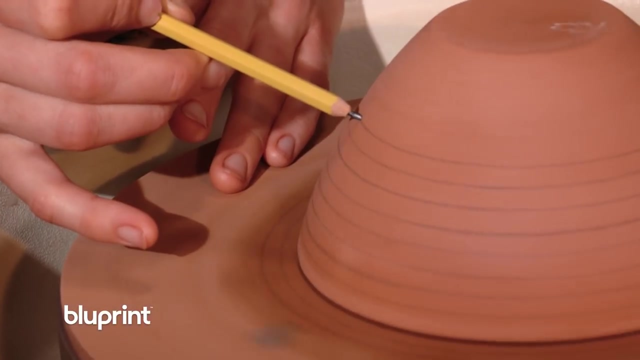 out with a pencil first. So I like to do a lot of my glaze prep on the wheel just so that I can get nice straight lines. I'm steadying my hand on the wheel as I do this. One great thing about using just normal graphite pencils is that the lines actually burn off. 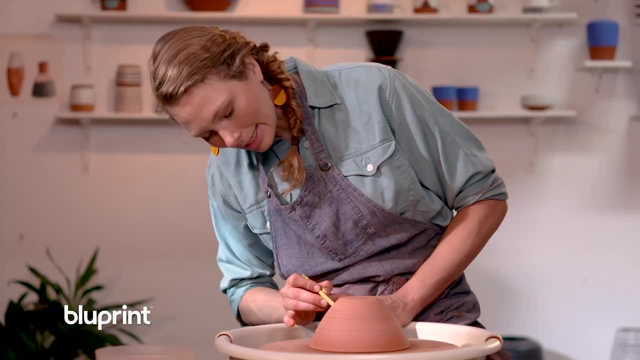 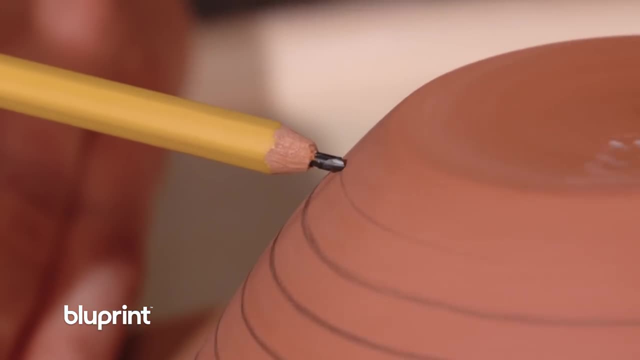 in the glaze firing. So you can map out all sorts of glaze ideas with a pencil and even just wipe them off and try again as many times as you want, without having to worry about it showing up on your finished piece. 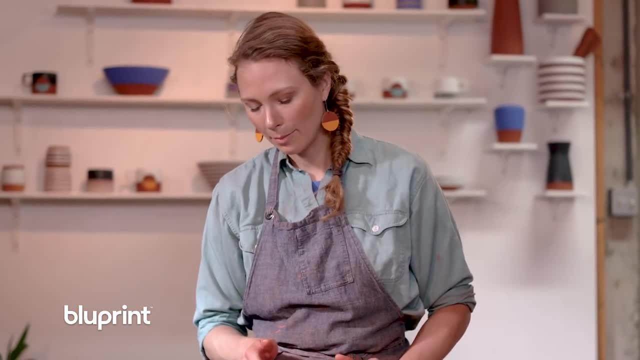 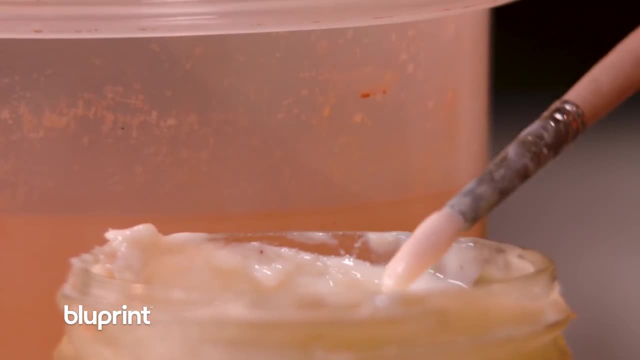 So now that I've mapped out all of my lines evenly up the side of my bowl, I'm going to go ahead and fill in every little bit, Every other line, with wax. I like to use a pretty nice brush for this, Something that doesn't have wispy hairs coming off the sides of it. that's going to get wax. 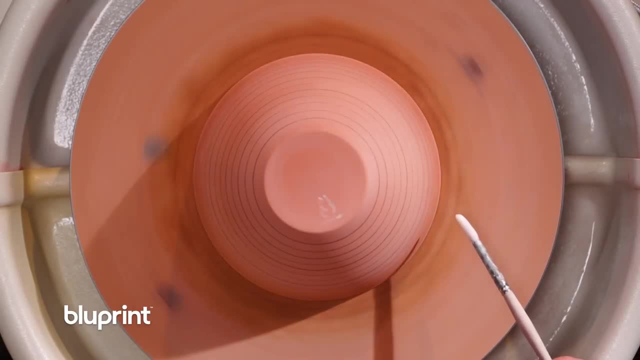 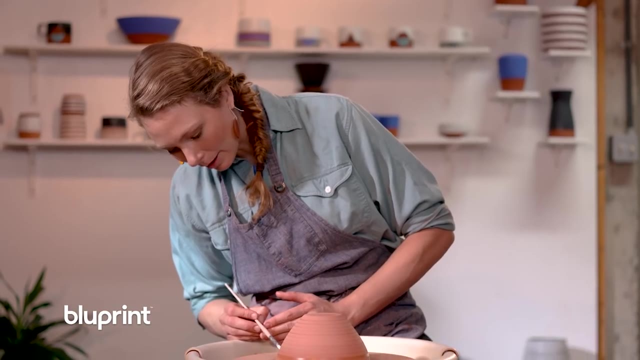 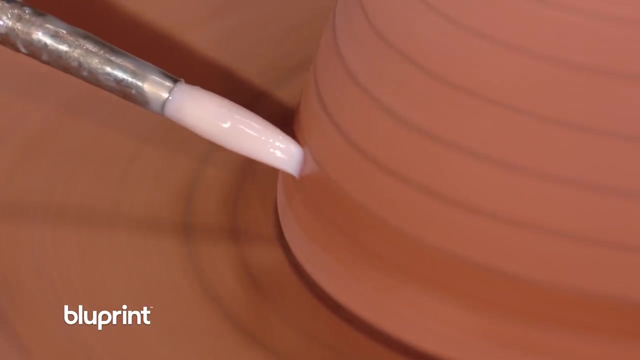 off to the side, where I don't want it. So, as I go, I'm just going to take my time. I don't want to fill my brush up with so much wax that it's going to drip out Again, just because I can't really remove the wax if it drips down the bowl. 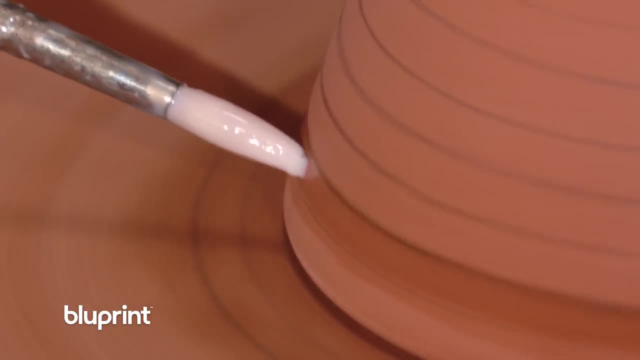 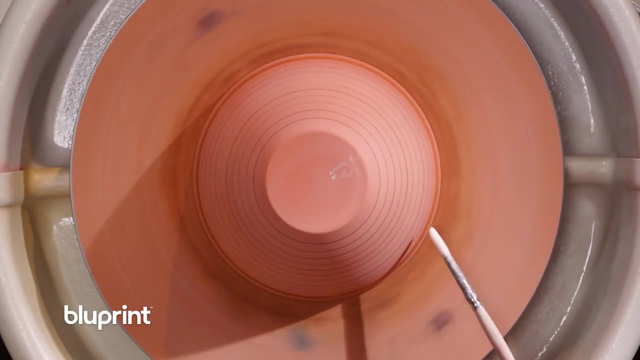 It's possible to try and sand it off If this happens, but generally it's best if you don't have any wax strips where you don't want them. So I'm just lightly painting on the stripes and I may go back once or twice during each. 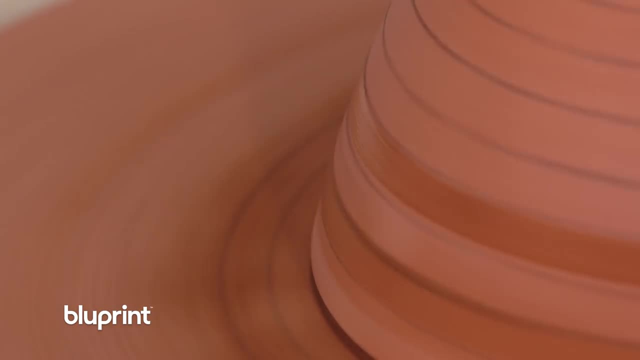 stripe to refill my brush with wax. I'm erring on the side of not enough wax on the brush rather than too much, just so I don't drip. I also like to come back a few times just to make sure that there aren't any little. 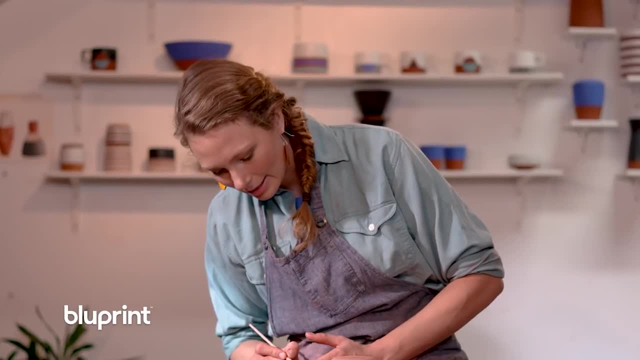 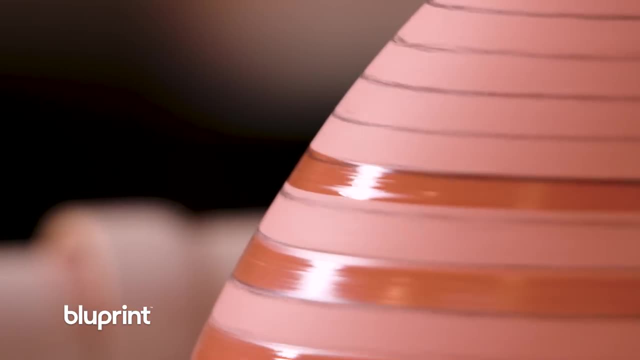 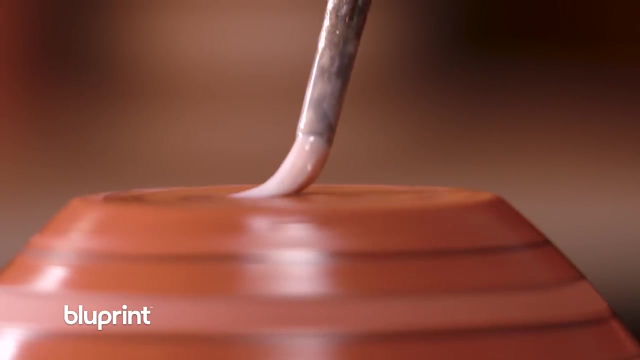 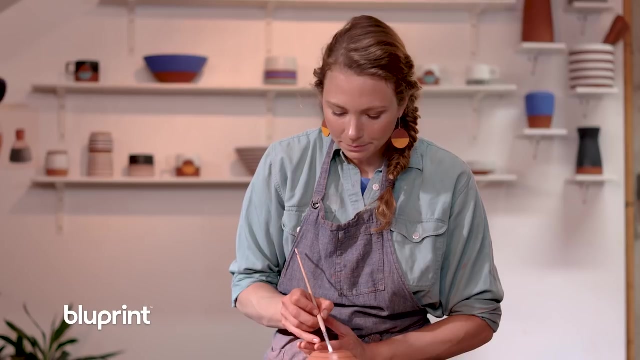 lines or areas on the stripe where I didn't get wax, because it's annoying to clean those up later. All right, so I'm going to go ahead and wax the bottom of my piece when I'm done as well, And this just leaves me at a point where the only parts of my bowl which I don't want to 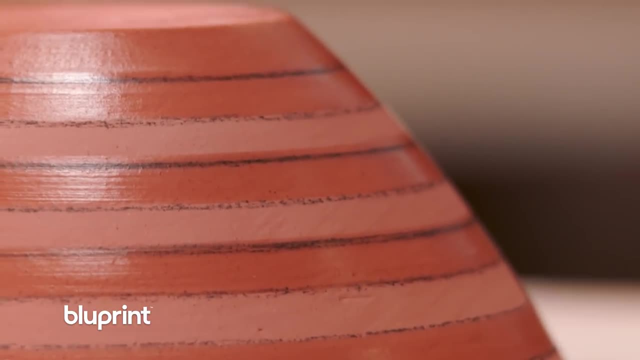 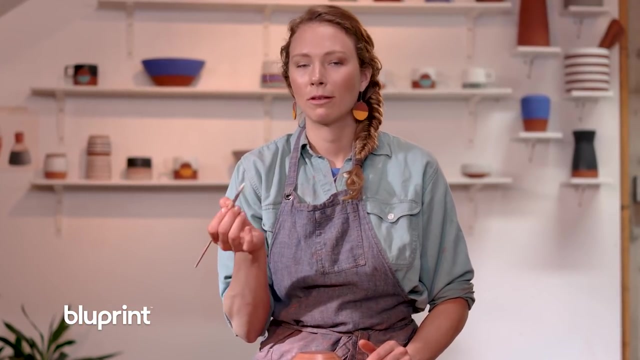 wax are parts that I want to have glaze on in my finished piece. So try some stripes and, if you want, go ahead and try just doodling with wax on your piece. It can be really fun to freehand patterns and designs with wax and watch the glaze bead. 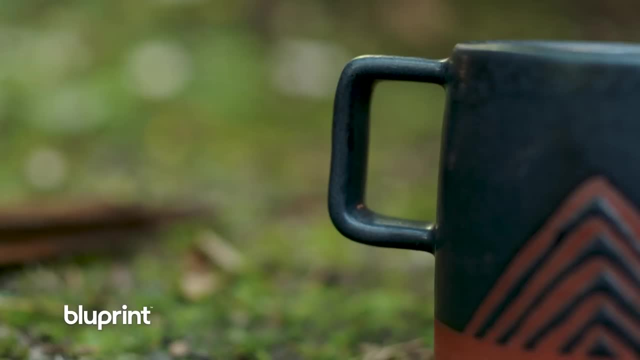 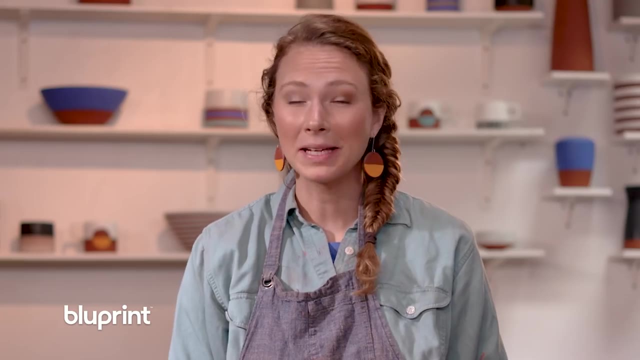 away and leave that image or those lines showing by the absence of glaze in your finished piece. So now that my piece is waxed, I do need to let it dry for probably an hour or two before I'm going to dip it in the glaze. 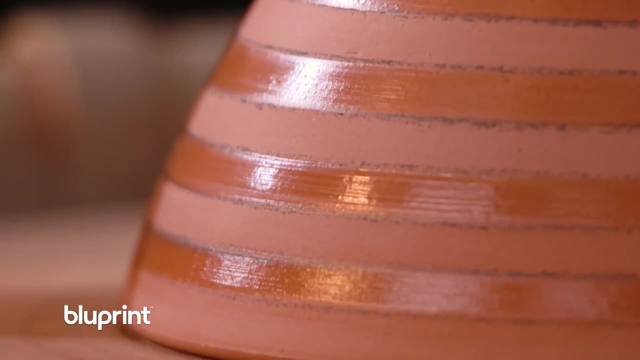 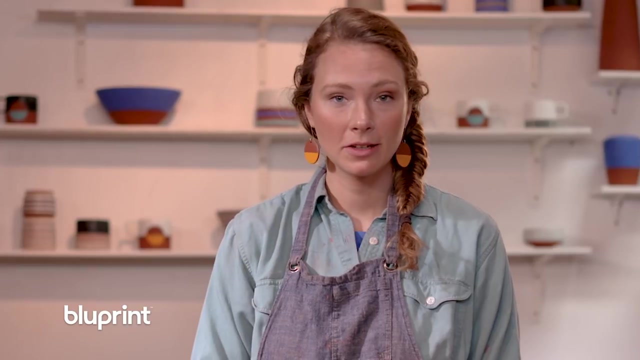 Because the glaze won't bead off well from the wax unless it's fully dry. So when you're going to move your piece somewhere to dry, just be sure not to touch the wax with your fingers, because the oils from your fingers will actually cause the wax to be. 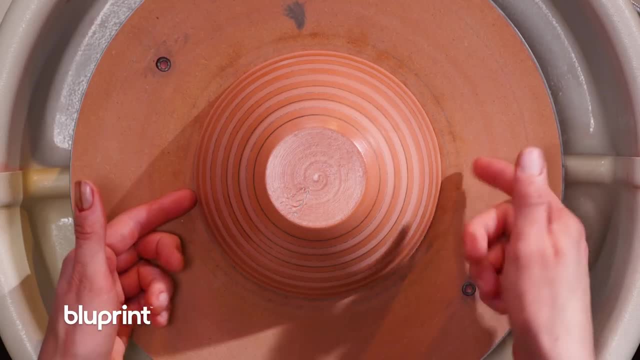 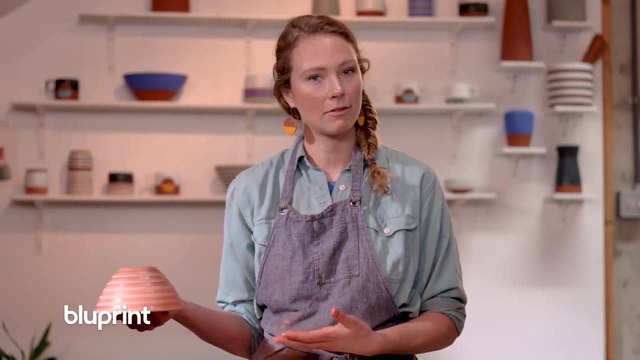 less resistant later. So in this case I'm just going to gently slide the bowl to the edge of the bat and pick it up from the very edge, And then I'll let it dry for about an hour or two before glazing it. 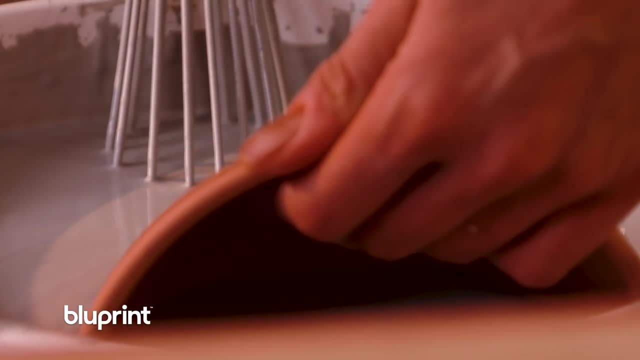 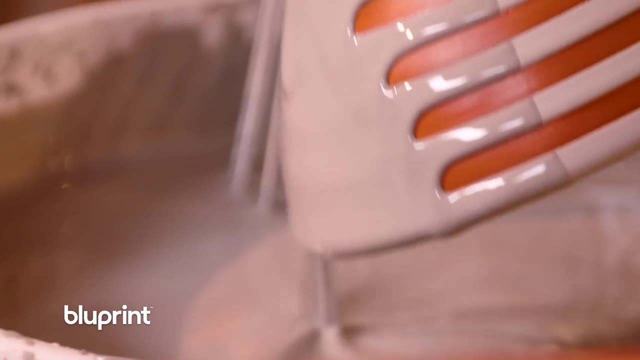 Once it's dry, I'm going to take my wax off. Once it's dry, I'll dip the bowl one half at a time, allowing it to dry in between. I'll clean up any drips as I go and make sure that the bottom of the bowl is free of any. 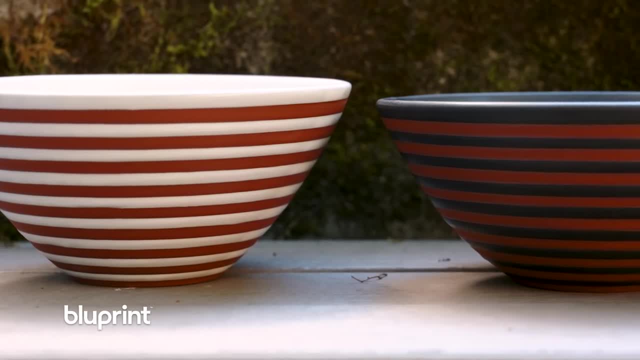 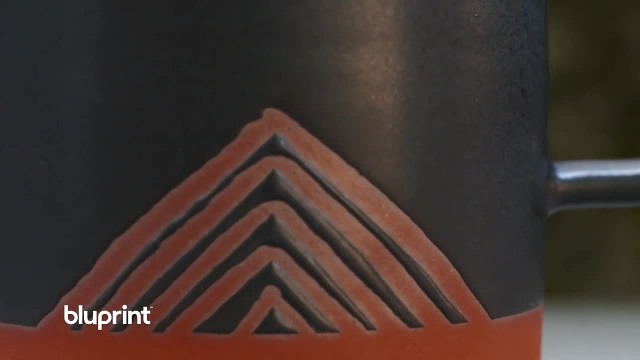 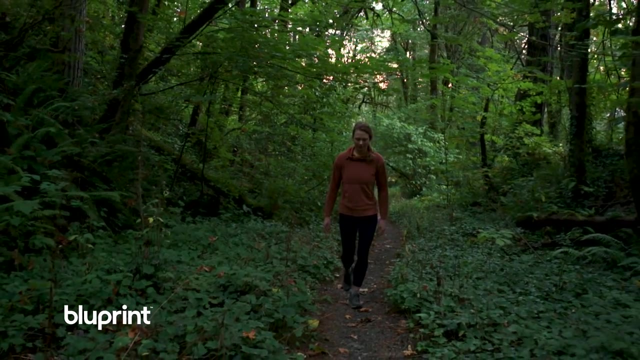 glaze before I put it in the kiln. I've always been attracted to really simple and bold designs that play with negative space and use classic shapes like circles and triangles, And I've also often found inspiration in the landscape around me. I'm from the Pacific Northwest. 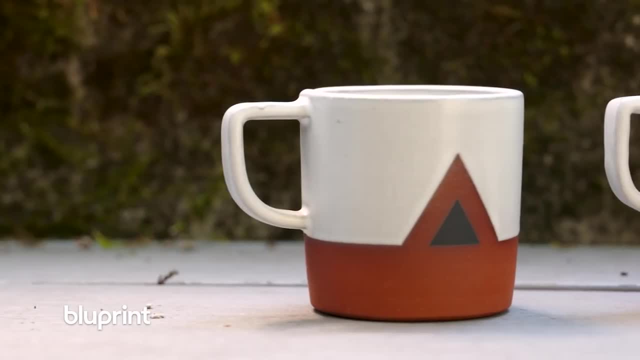 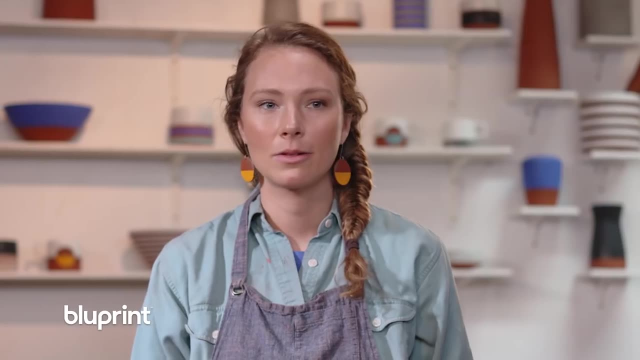 And I spend a lot of time in the Midwest, So today I'm going to show you my mountain mug. I like to use vinyl for a lot of my designs because it enables me to make multiples of the same shape. So I can go on to the computer, design my shapes and actually have them cut out by. 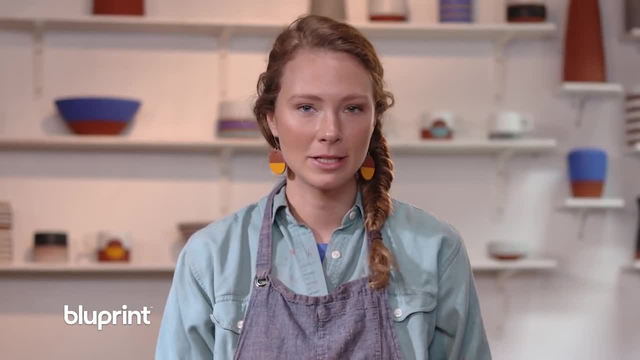 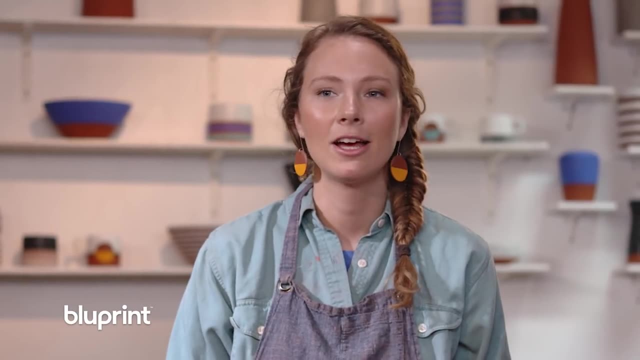 a machine that cuts vinyl. Vinyl is basically like a sticker material, but it's not at all necessary. If you have masking tape and a pair of scissors, you can mess around with this technique just fine, Or even an X-Acto knife might be really helpful. 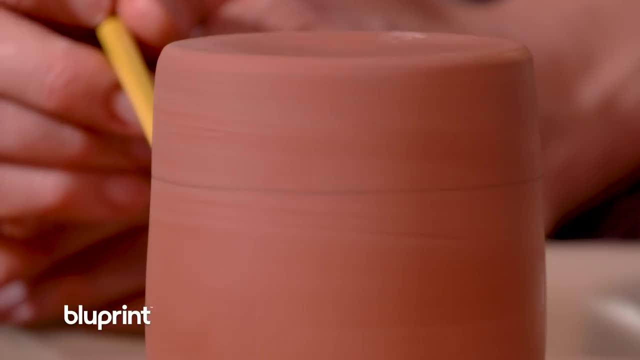 I start by drawing a pencil line about an inch up from the bottom. I'm going to start with the bottom, Giving me a place to line up my vinyl or tape. Then I add my vinyl triangle, centered on the front and back of the mug. 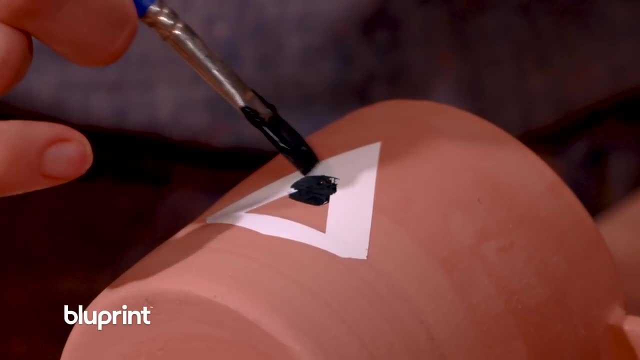 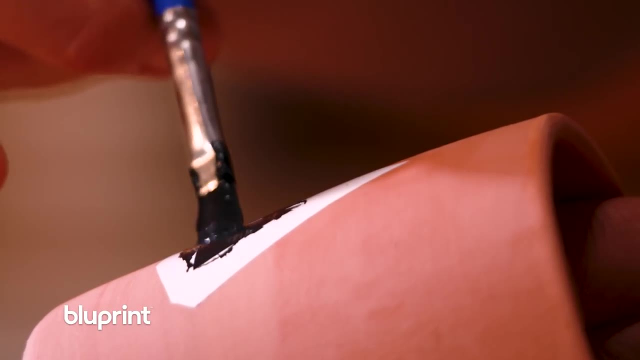 The next step is to paint underglaze on the interior of the triangle. I usually do a couple coats of underglaze, depending on how thick it is, Just until it looks opaque. It dries pretty quickly, so it's easy to do a few coats in a row. 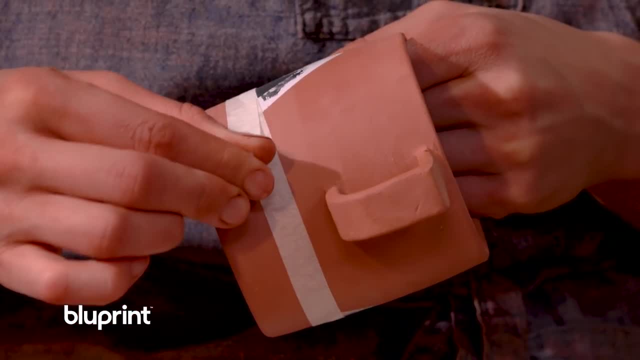 Once the underglaze is dry, I add a strip of tape along the bottom of the mug in line with the underglaze triangle. I then paint wax on the triangles so that they'll be protected when I dip the mug. Let it dry for at least an hour. 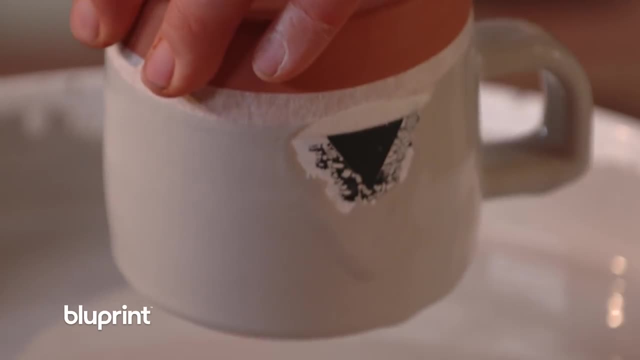 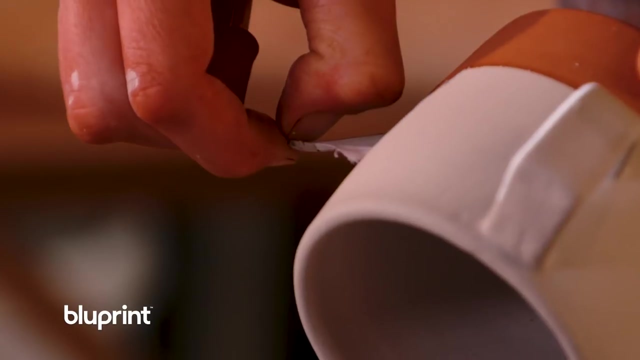 I'm going to start with the bottom. Let it dry for at least an hour or two. Once it's dry, I dip my mug with my hand using the pitcher method that I showed you earlier. Once you peel away the vinyl and the tape, your mug is ready to fire. 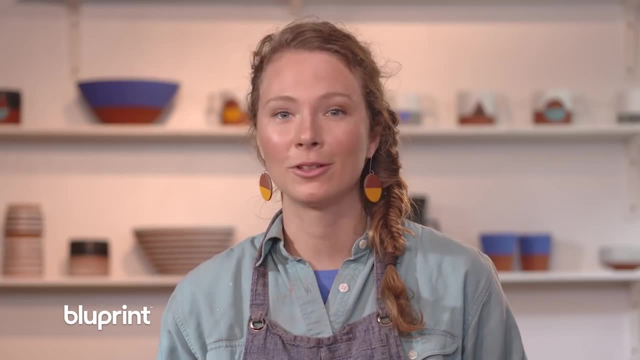 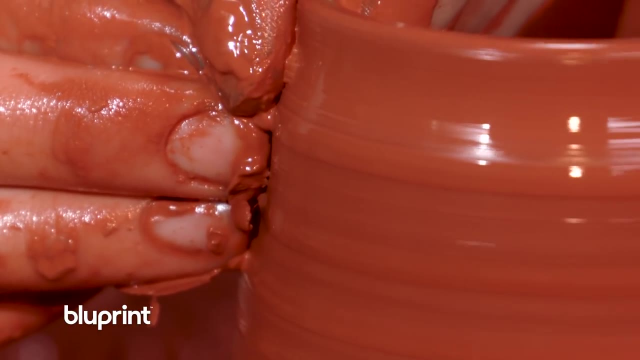 I find the process of working with ceramics so fun and fulfilling and full of possibilities. Over the years of learning this craft, I've gone through so many phases and aesthetics and different styles and it's been so fun to have the opportunity to just explore the 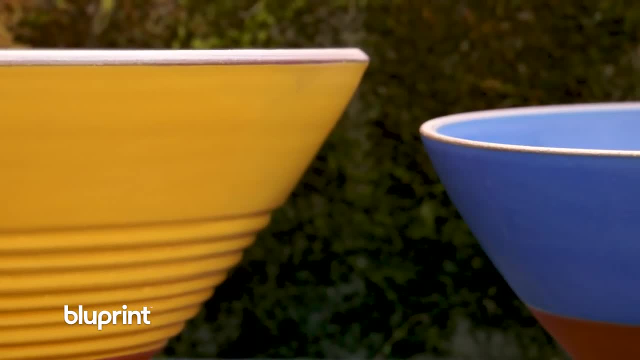 material. I hope I've been able to leave you with some ideas and techniques to get you started in the process of finding your own style.